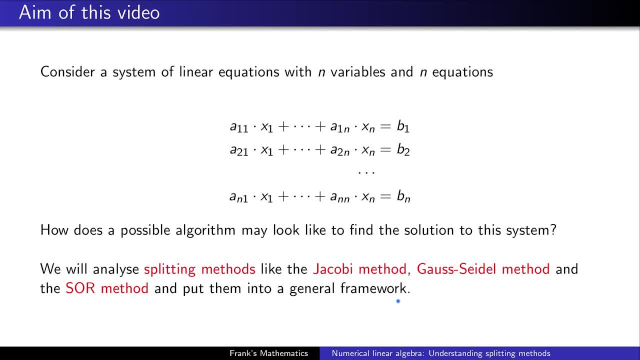 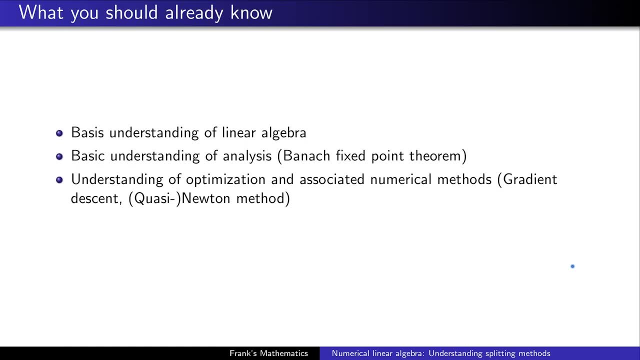 where we will start with the more general framework and then come to the more special parts. so we will put them in the general framework which helps them to analyze such methods. Since this is a more advanced method, more advanced video, you should have a basic. 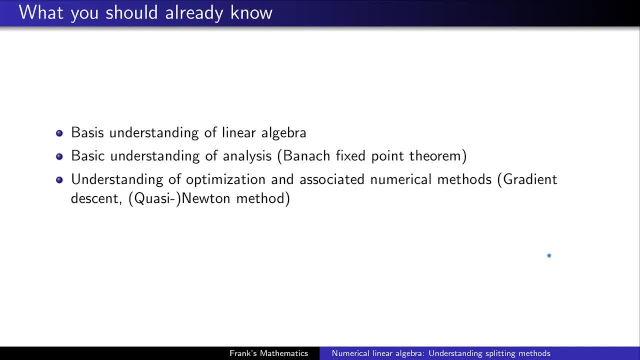 understanding of linear algebra. You should have heard analysis, one or maybe two, so you should know what the Banach fixed point theorem is and how to apply it. And it is good to know stuff about optimization and its associated numerical methods like the gradient. 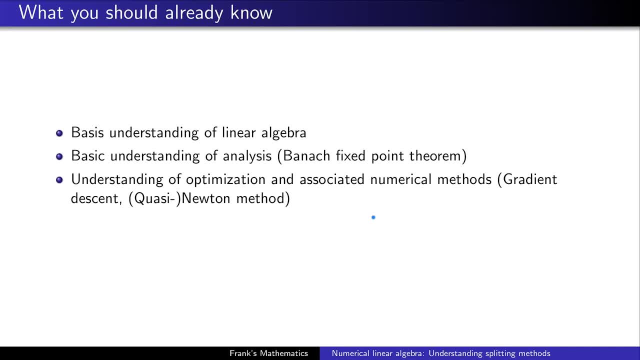 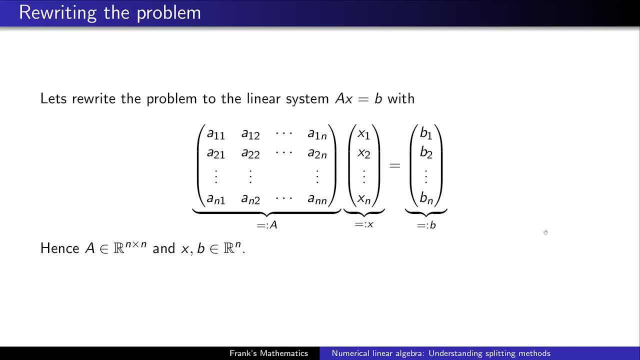 descent method or the quasi-Newton method. To start, we are going to rewrite the problem, so our n linear equations. they of course can be reformulated as a matrix vector multiplication. so let's define our matrix a to be the matrix of the coefficient you've seen in linear equations. 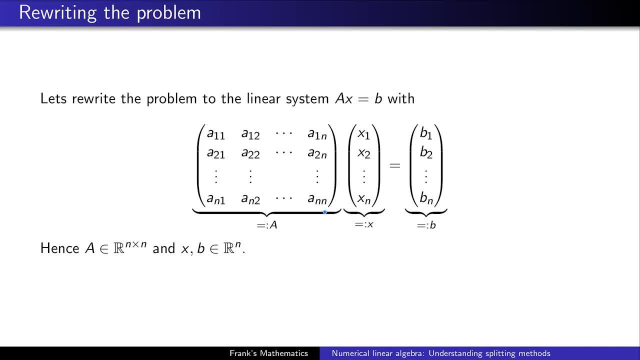 so it contains just a11, up to a and n. x is the vector we're looking for, and b contains the coefficient of the right-hand side. And then, of course, we want to form a matrix vector which is a vector故. Wouldn't we call it a vector? 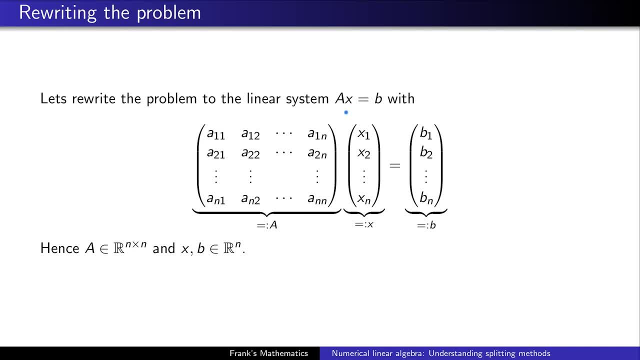 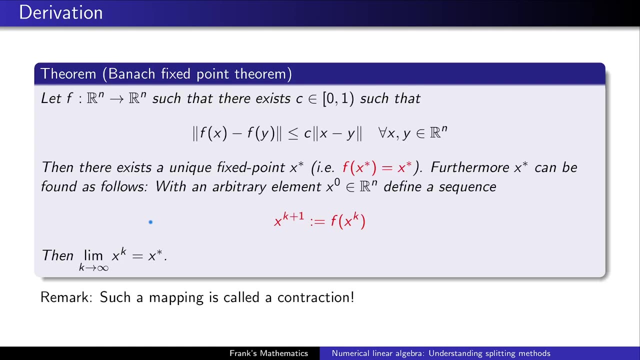 And of course the n linear equations can be rewritten as a matrix vector. multiplication a times x equals b, with a being the quadratic matrix. I've mentioned in the introduction that we are going to need the Banach fixed point theorem. This might look a bit arbitrary here, but you'll see in a moment that this is a very 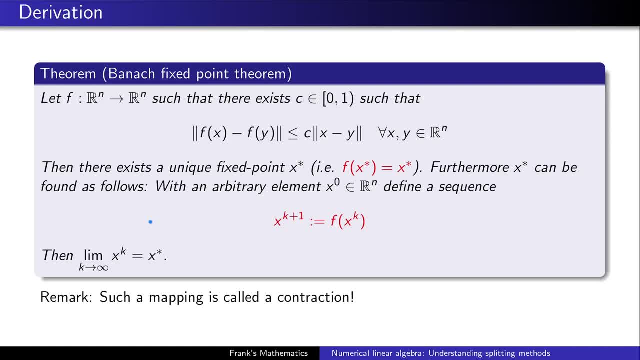 useful method and a very useful technique to analyze such splitting methods. Let's take a look at this theorem. We'll need a function f going from the space Rn to Rn in such a way that the difference of the mapping so f of x minus f applied to y in the norm of Rn should be less or. 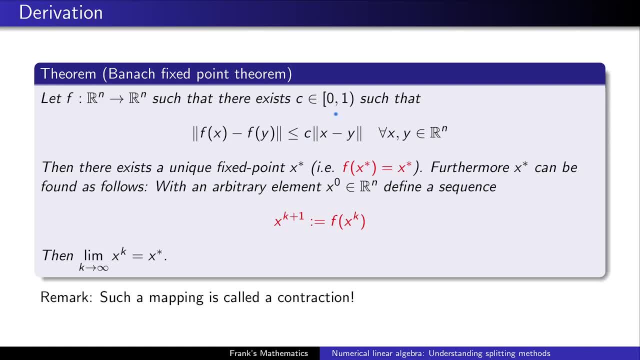 equal than a constant c, And it's important that c is the coefficient between 0 and 1, and 1 is not included- times the difference of x and y. If this equation holds for all x And for all y in the space Rn, then such a mapping is called a contradiction. 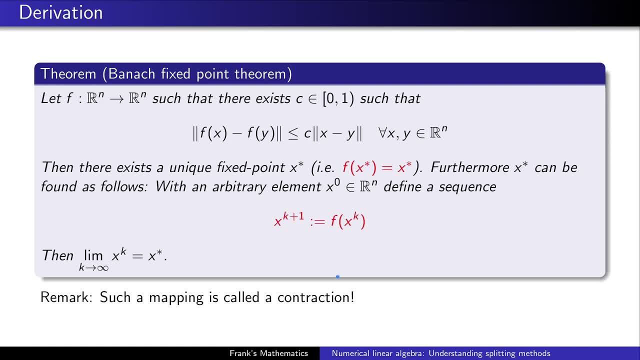 And this contradiction can be used to actually prove that there exists not only a fixed point, but also a unique fixed point: x star. So being a fixed point means that f applied to x star is equal to x star, So this is a very strong condition. 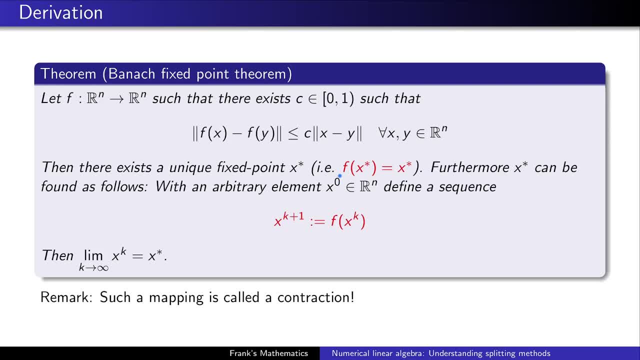 And furthermore, we do not also know there exists a unique fixed point. we also know how to compute it. This is a very useful technique. Let's start with an arbitrary element- x0,, which is randomly chosen, And we define the following sequence: 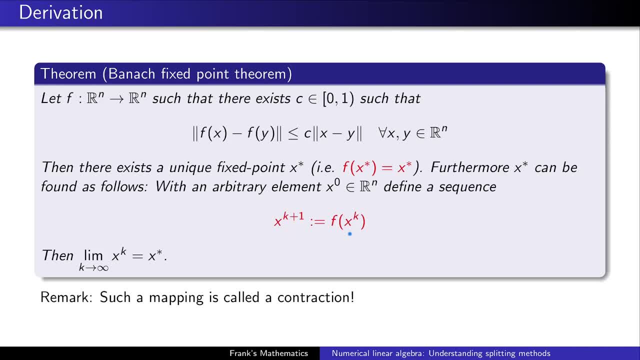 So xk plus 1 is f applied to xk, Then we know that the limit of this sequence is x star. So this is a way to actually find the fixed point, And if we are now able to reformulate our problem to a fixed point, then we can actually 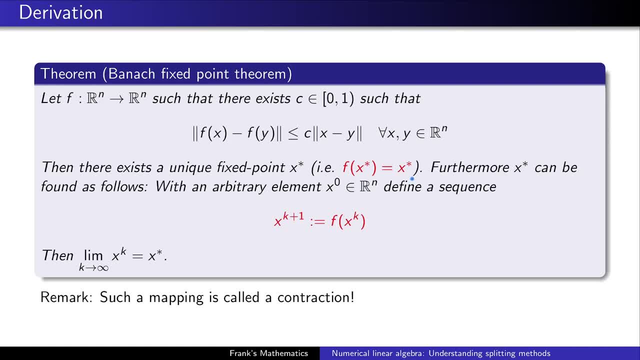 find the fixed point. And if we are now able to reformulate our problem to a fixed point, then we can actually find the fixed point. And if we are now able to reformulate our problem to a fixed point, then we can actually find the fixed point. 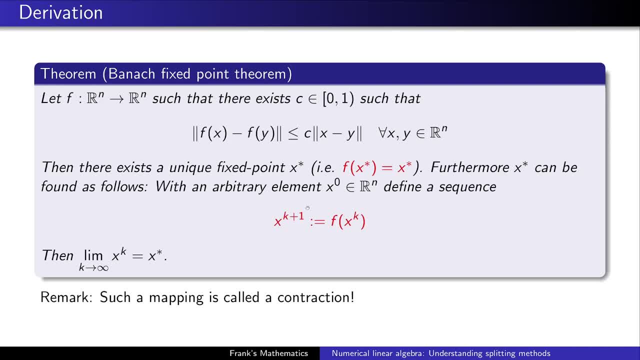 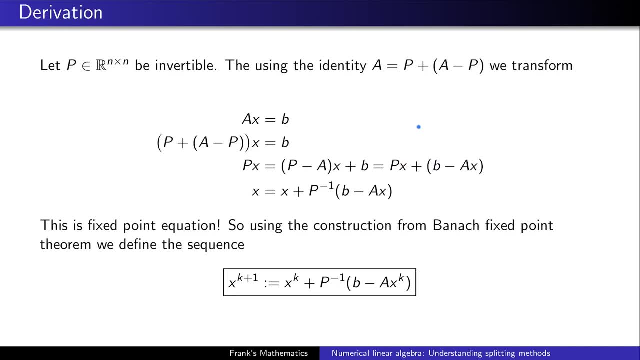 And if we are now able to reformulate our problem to a fixed point, then we actually can compute the solution to our problem just by applying this recursive iteration here, And this is exactly what we're going to do. now, of course, We start with an invertible matrix. let's call it p. 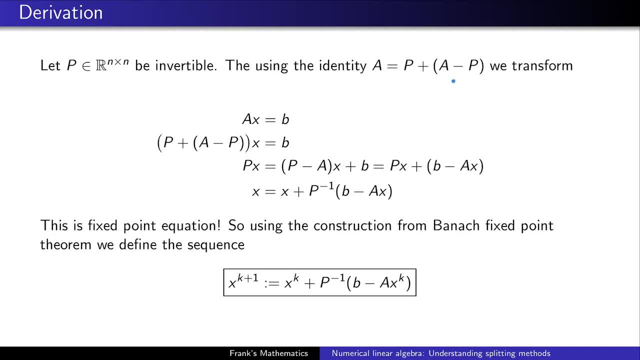 Then of course we know that a is p plus a minus p, just p cancels out. Might look very stupid here, but in fact let's transform our system: a times x equal b By replacing a with p plus a minus p. 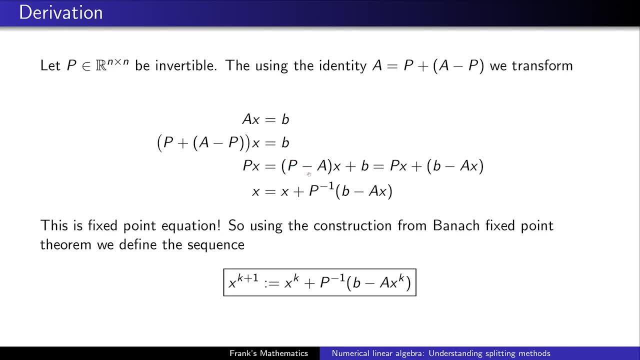 Bring a minus p to the other side. so it's there: p minus a times x plus b. Reformulate some terms so we have: px is px minus b minus ax. And now we know that p is an invertible matrix, so we can bring p from the left-hand side. 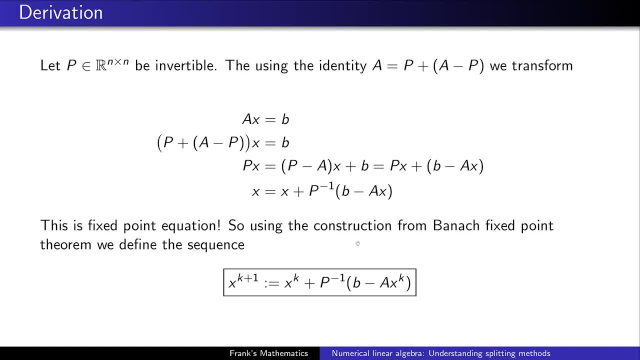 to the right-hand side of our equation And we will end up with x being p. And now we know that p is an invertible matrix, so we can bring p from the left-hand side to the right-hand side of our equation. We have x plus p minus 1, so the inverse of p times p minus ax. 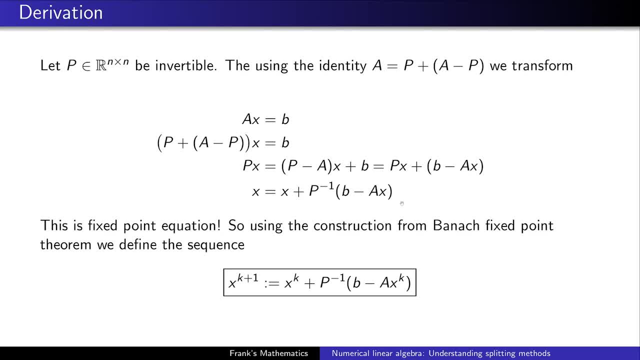 And of course this is a fixed-point equation, because x is here and here is some function applied to x And using the construction from the Banach fixed-point theorem, we know that the following sequence: so if you call the right-hand side here f, then we know that it is the: 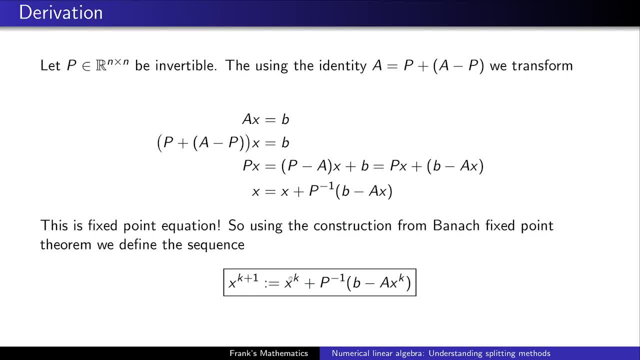 sequence defined by xk plus 1 equals f. We know that the sequence defined by xk plus 1 equals f. We know that the sequence defined by xk plus 1 equals f. x which is f, which which is xk, plus the inverse of p times b minus ax. this under, if this is a. 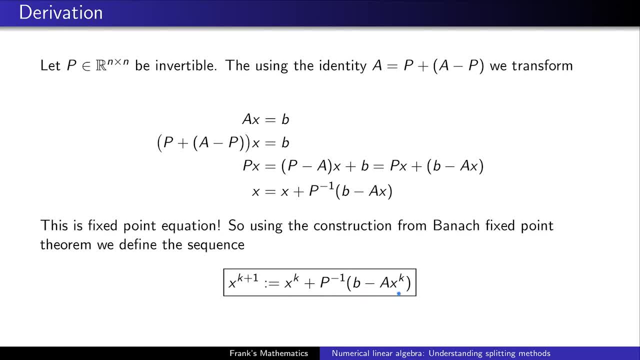 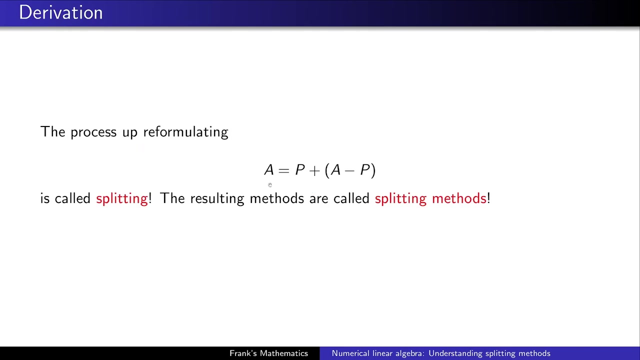 contraction. of course, this will converge to our solution of um of ax equals b. so this is a very good starting point to get a method out of it, and this is exactly what we will use throughout this video. why is it called splitting method? because the process of reformulating a equal p plus a. 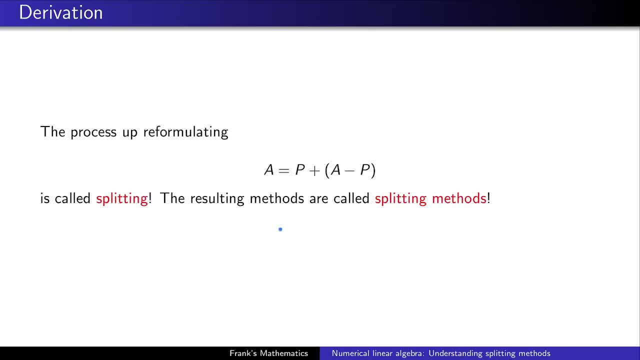 minus p. this is called splitting. so we split the matrix into two parts, so basically p, and well, what's ever left? so a minus p. this is called a splitting for obvious reason, and the resulting methods are therefore called splitting methods. and the trick is now to choose p. 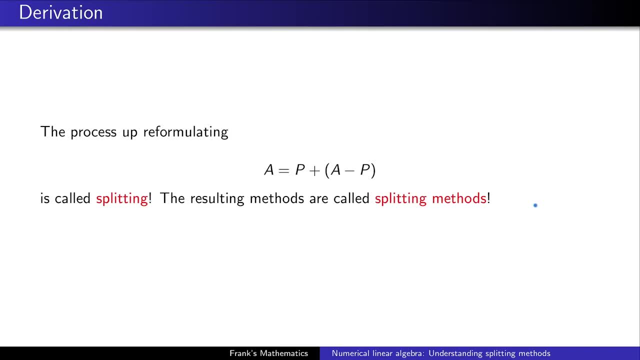 in a suitable way to get some nice methods out of it. Just a small remark: You can see here the splitting method. again, We can reformulate this a little bit just by introducing the variable RK, which is just B minus AX. If RK is zero, then we know that B is AX. 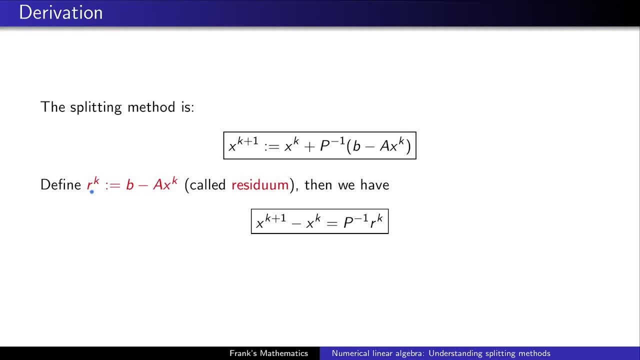 So this- that's why I called our, that's why our call RK is called- is the Residuum, And if we reformulate this a little bit, then we know that XK plus one minus XK is actually P minus one times the Residuum. 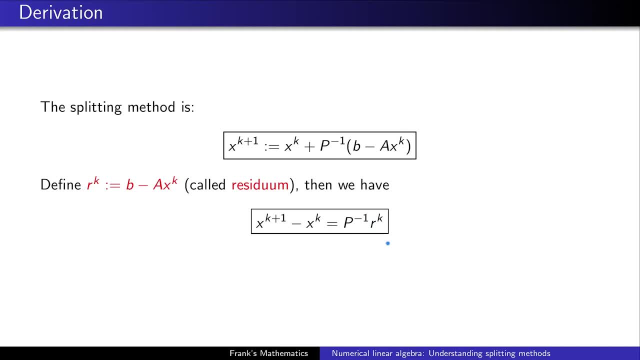 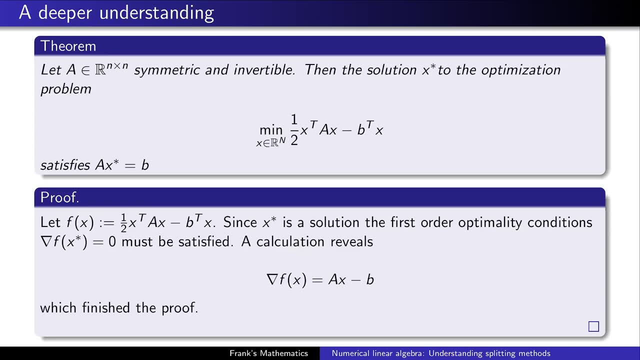 So the trick is to find a suitable P, such the Residuum goes to zero. Before we start with some specific examples of how to choose the matrix P, let's get a little bit deeper understanding what's actually going on here. So for the following theorem, 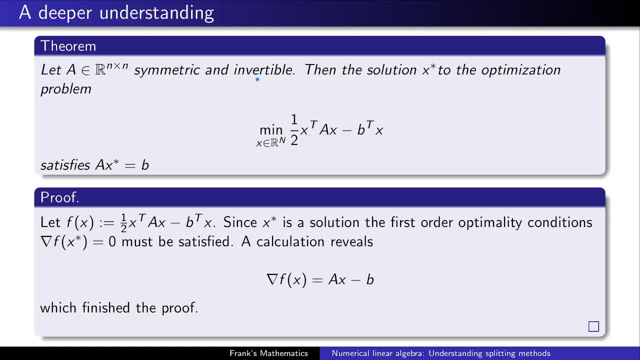 we assume that A is a symmetric and invertible matrix, Then we know that the solution X star to the optimization problem. we minimize X, transpose AX minus B, transpose X, which is a real number. It's a real number here That this solution satisfies. AX star equals B. 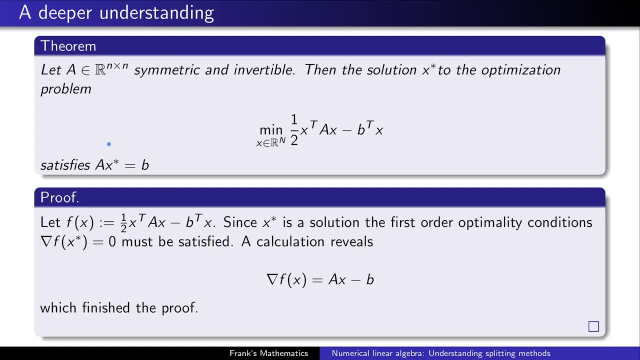 So this is the system we're looking at. We want to find a solution, for The proof is quite easy. Let's define this thing here. at BFX, We know that X star is a solution, So we know that the first order optimality conditions. 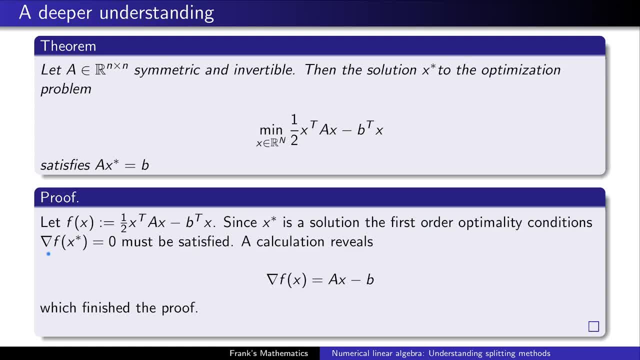 which are just F. prime at X star equals zero, or the gradient of F must be zero at this point. This must be satisfied, And if you do a quick calculation using that A is symmetric, we know that the gradient of F is just AX minus B. 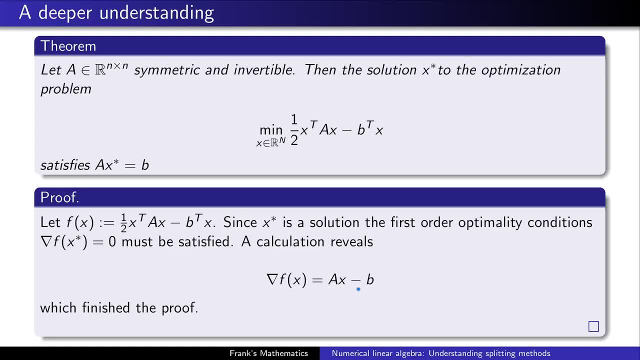 And if the gradient is zero and then A of X, then AX minus B must be zero, And this finishes the proof. In fact, this is not all. This is also a necessary condition. This is also a sufficient condition just because this is a convex problem. 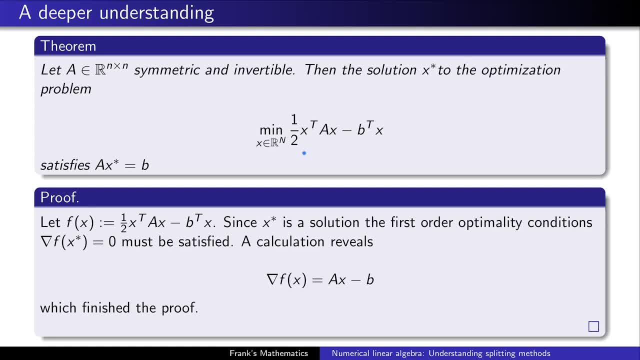 which means that the first order optimality conditions are also sufficient. Just as a small remark, we only need the necessity of the first order optimality conditions. So throughout the next slides, keep in mind that our system can be formulated as an optimization problem. 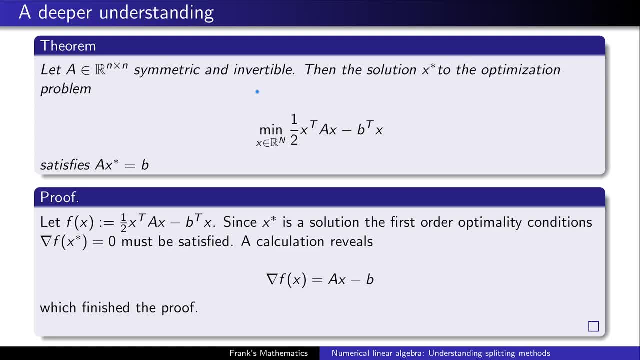 Or to be more precise, as the first order optimality conditions for the minimization problem. But if you think about how to find solutions of optimality conditions, you usually search for points which satisfies the first order optimality conditions. And if we go a little bit deeper, 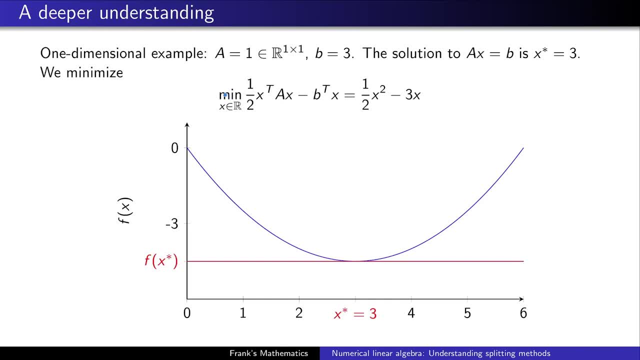 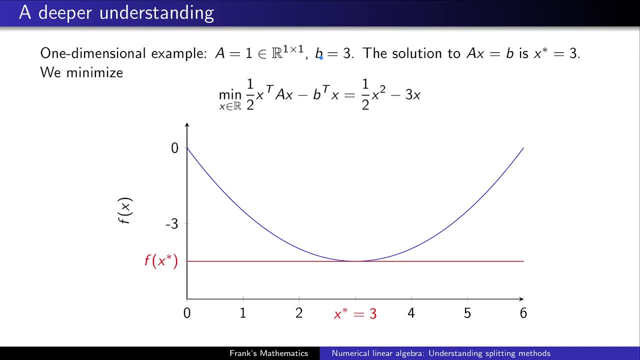 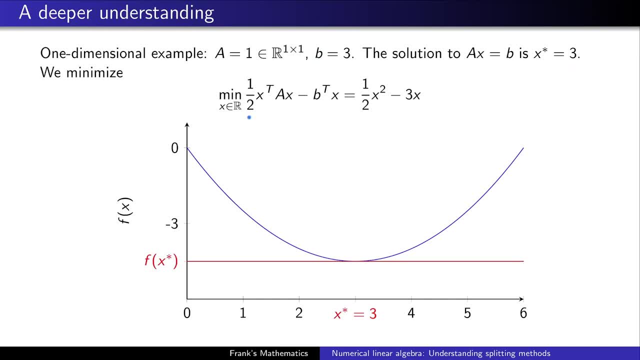 X star equals three, of course, And the thing, the function we want to minimize, looks like this: So this is one half X times X minus three X, And if you plot this in a graph, the blue line is F of X. 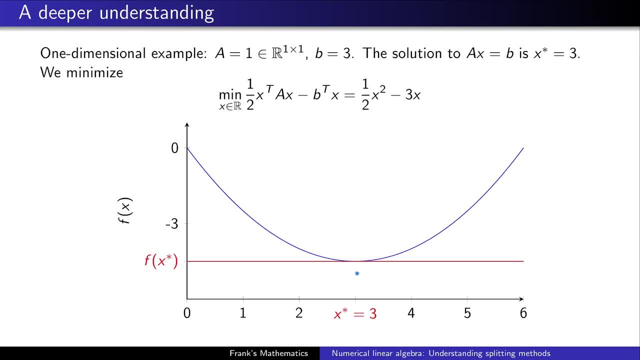 So the blue line is this term here And the minima. the minimum of this function is of course by construction. we just proved it at the point X. star equals three. So this kind of is a visualization of the optimization problem. 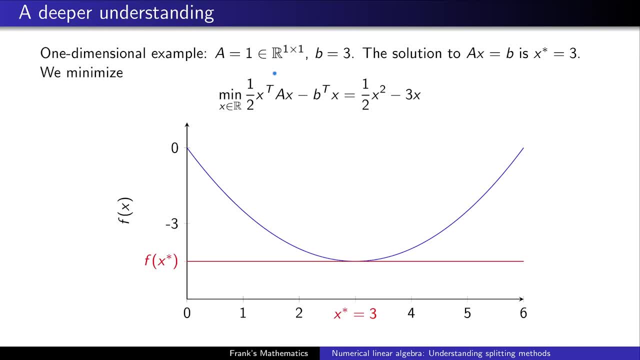 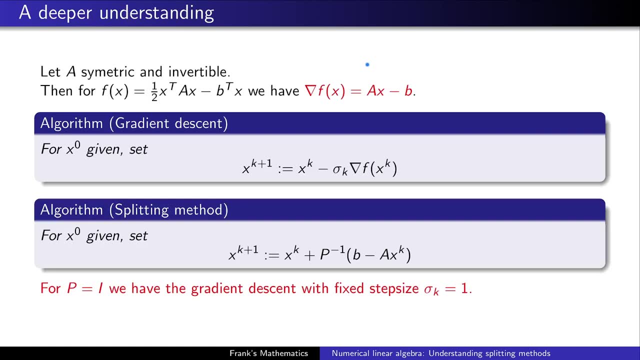 But of course we are gonna do it in more dimensions, but therefore it's harder to visualize it. I already mentioned that we need a gradient descent. So why do we need a gradient descent? This is quite easy to see, So let's hop into the gradient descent. 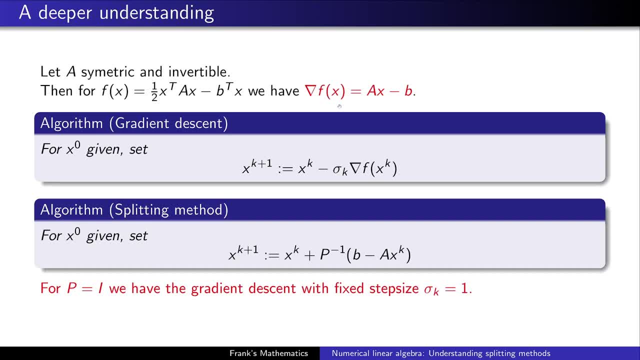 As already known, we know that the gradient of this function F here is AX minus B And the general gradient descent looks like this: We start with X, zero given, and then we compute: X K plus one is X K minus a correction term. 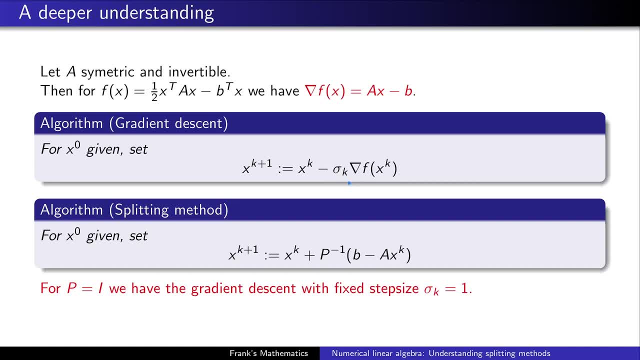 And the correction term is given by some step size. theta times the gradient of F, X in the negative direction. So we go into the direction of the steepest descent. Recall that the gradient points into the direction of the greatest essence, So putting the minus in front of it. 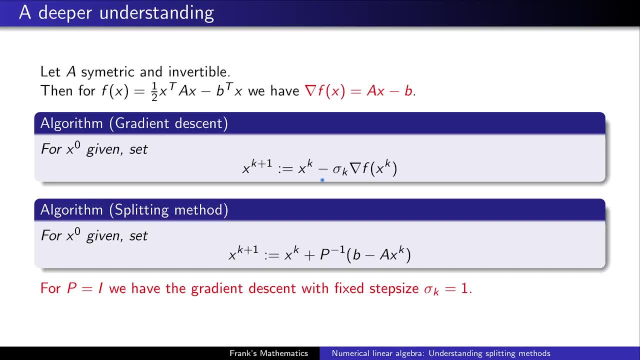 gives us the direction of the greatest descent, And this actually looks very similar to our optimization at our splitting method, which you can see here. If we choose P to be the identity, well, and using the gradient of this function here as AX minus B, we know that these two terms 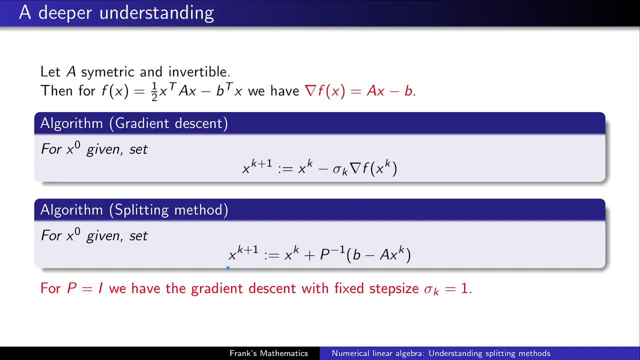 are actually the same. So what does this mean? This means that for the specific choice of P equals A and P equals the identity, the splitting method or the restarting method can be interpreted as the gradient descent with fixed step size equals one. for this optimization problem, for this function here. 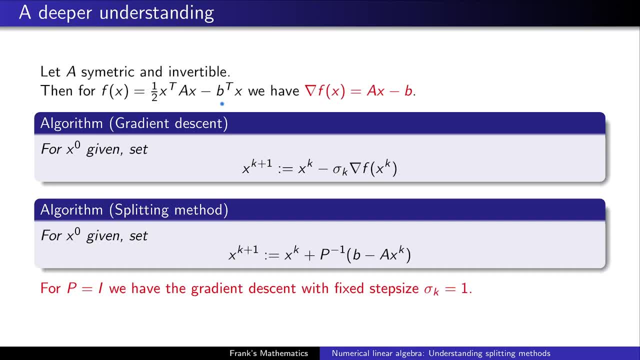 And this is quite interesting because now we have put two completely different methods into perspective. I mean, the derivation was completely different. I mean the gradient descent is well, if you want to put it that way, is an algorithmic interpretation going into direction. 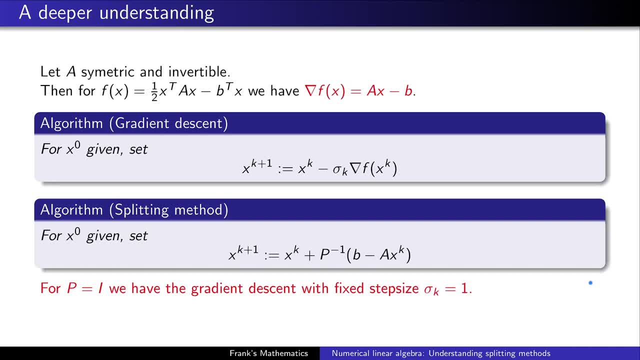 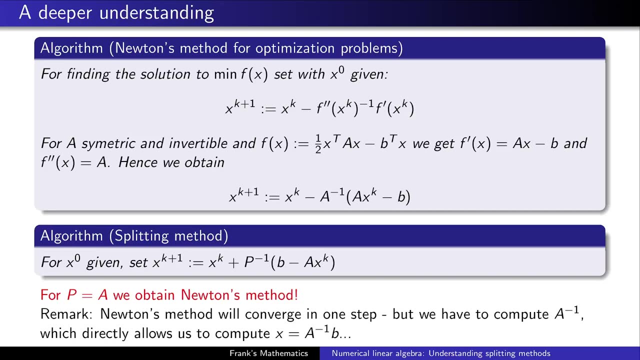 of the steepest descent. while the splitting method more or less can be constructed using the Banach fixed point theorem and some splitting, But still for the specific choice they are the same. Before we move on with the splitting methods, let's quickly take a look at Newton's method. 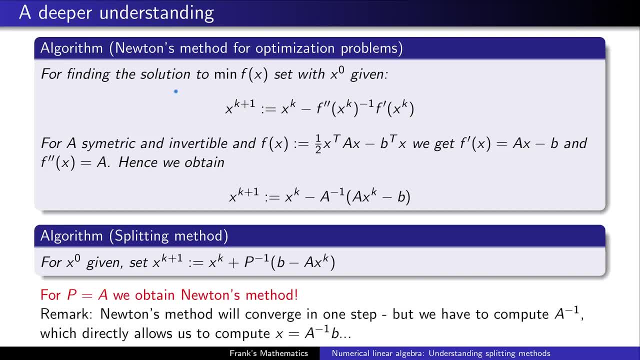 for optimization problems. So we want to find the solution to minimizing f of x. To do so we start with x0 given and compute, index, iterate xk plus 1 to be xk minus, the inverse of the second derivative of f applied at xk. 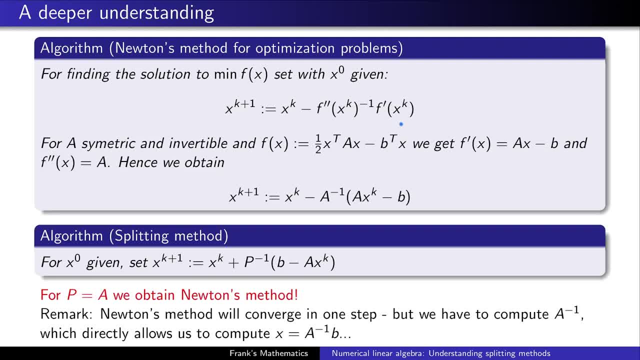 So f prime of xk times f prime evaluated at xk. For our specific problem we choose f to be again ax minus bx And we compute the first and second derivative. You can see them here. So f of x, f prime of x, is ax minus b. 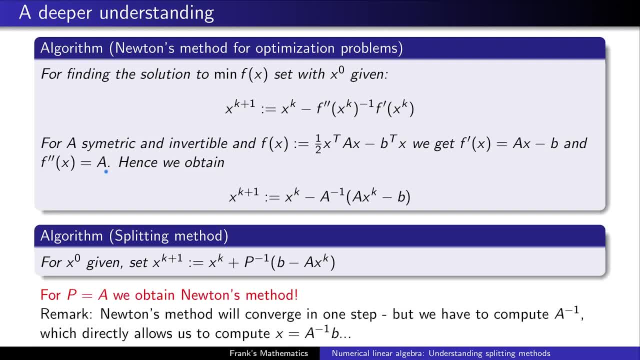 And the second derivative is just a. If you plug in these values into the Newton's method in the general formulation of the Newton's method here, well you end up with this formulation here. So xk plus 1 is xk minus, inverse of a times ax minus b. 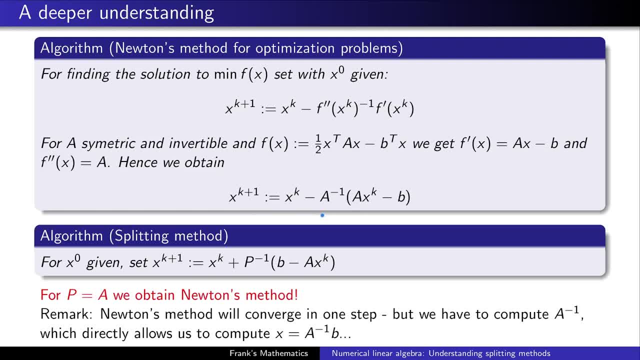 Can we put this into our general framework for the splitting methods? Of course we can. You can see it here. And if you choose p to be equal a, we obtain Newton's method. Let's just see it here. However, this is of course I mean. 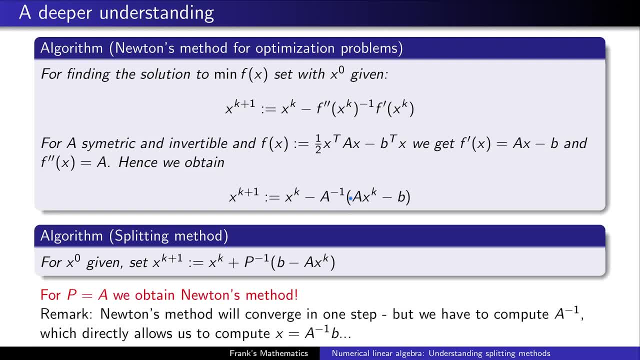 applying Newton's method for a linear system is quite an overkill, For two reasons. The first reason is, of course, Newton's method will converge in one step, which is super nice, But second, we have to compute the inverse of the matrix A. 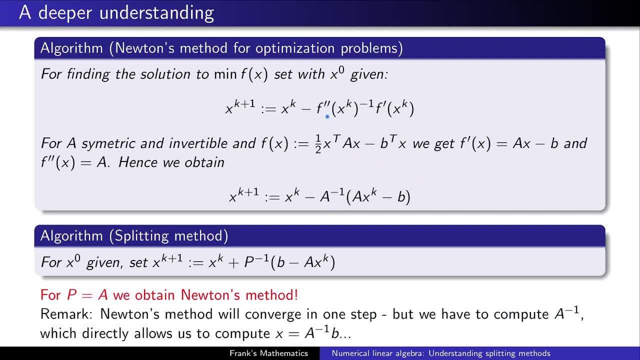 because we'll need the inverse of the second derivative. you can see here. But if you have to compute the inverse of the matrix A, well of course we can just compute the solution to our problem directly. So that's nah, It's quite an overkill. 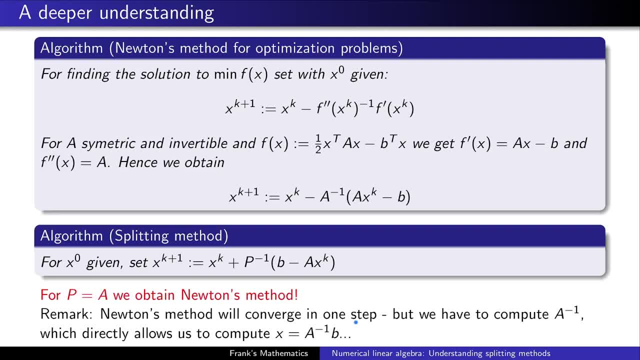 I just want to put it here into perspective. We have now seen two extreme values for p, So we have two extreme values for p. p chosen to be the identity will give us the greatest descent method. p to be chosen, the matrix A will give us Newton's method. 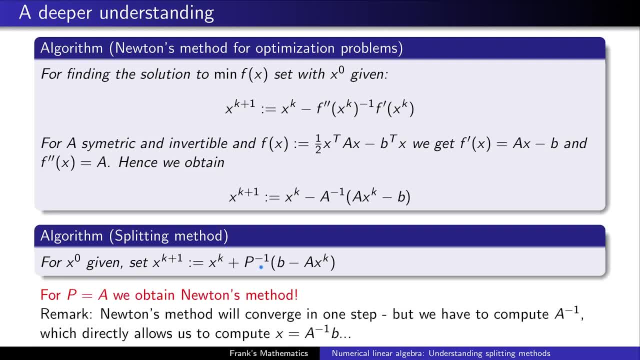 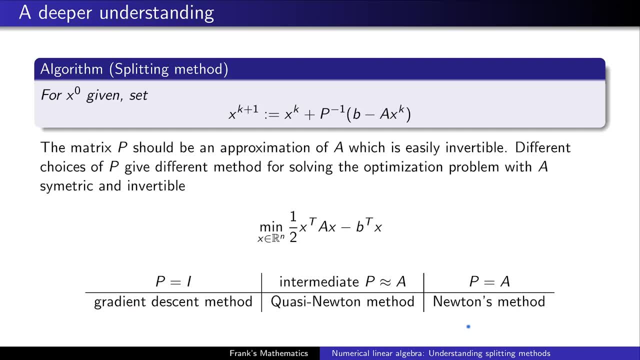 What if we choose p to be something in the middle? This is the idea of this slide here, So let's start with the table here. Here you can see what happens if we choose p- p to be different values. The idea is the matrix p should be a good approximation. 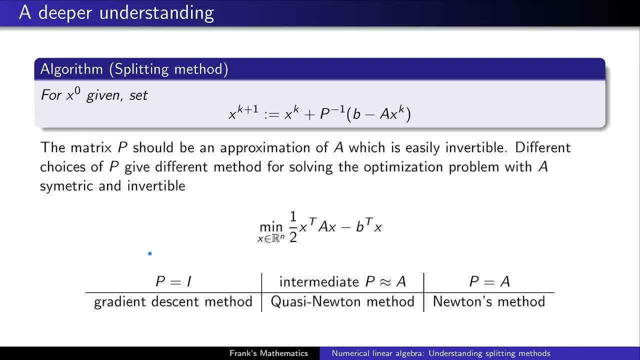 of the matrix A with the property that it is easily invertible. So if you choose p in a different way, this will give us a so-called quasi-Newton method. Let's take a look at this table here. If you choose p to be the identity, of course 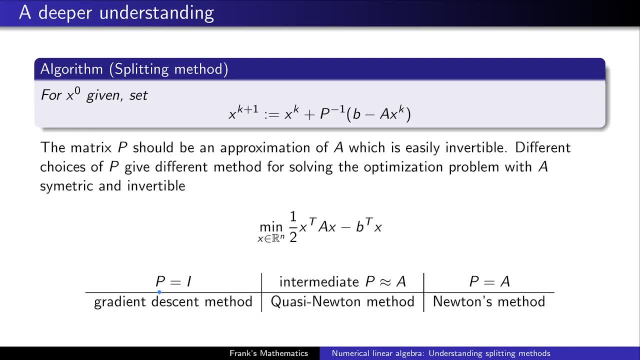 then the matrix p is super easy to be inverted, But it's not. But it's a very poor approximation of A. On the other hand, if you choose p to be A, this is a very, very good approximation. In fact, this is the best approximation of A. 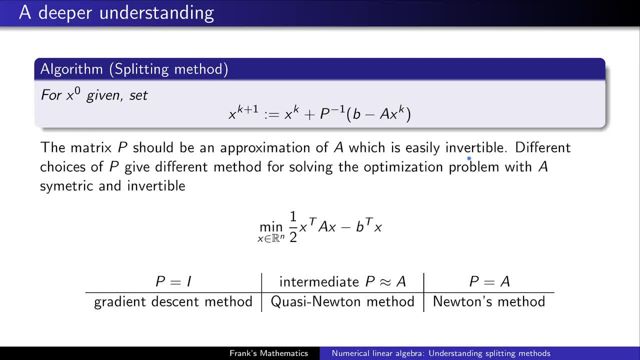 However, it might be easy to invert So for something chosen in the middle, whatever this means. this will be made clearer on the next slide. we'll end up with the quasi-Newton method for solving this optimization problem, And this is a very good. 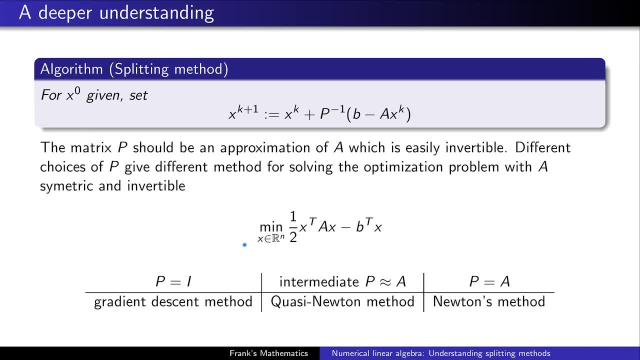 Or in my eyes it's. in my opinion, this is a very good overview, a very good interpretation, in fact, of the splitting method, to interpret it as optimization methods or algorithms for solving optimization problems. And in the following we will now get into some actual methods. 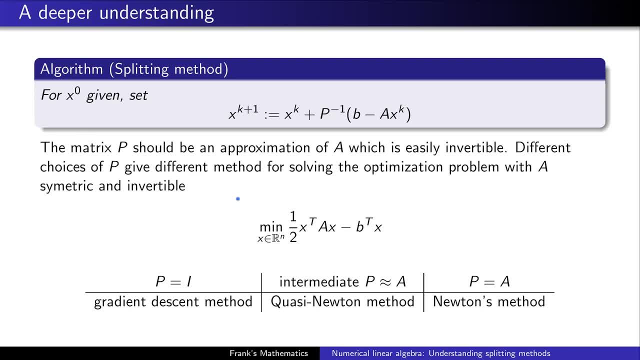 because nobody will compute the splitting method in such a way, Because then you have such a matrix vector formulation, you have to invert p. This is not suitable. But in the following I will present you three different methods which are splitting methods. 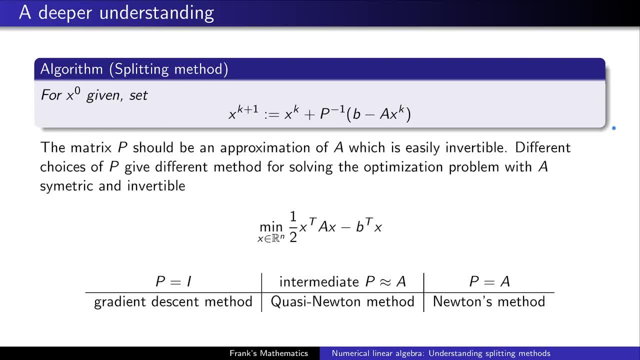 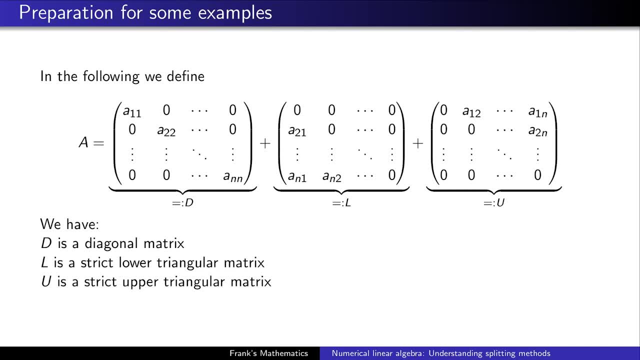 And I will show you how to put them into our general framework For the derivation of the examples. it's very useful to have the following splitting of the matrix A. So we split A into three different parts. So the first part is called the matrix D. 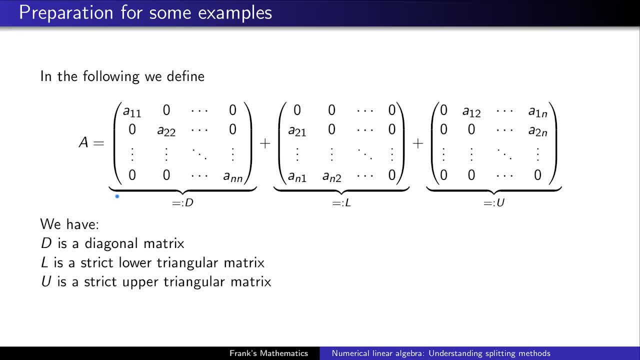 This is just the matrix containing all the diagonal elements. So D is just a diagonal matrix. L is a strict lower triangular matrix. It contains all the elements which are below the diagonal, And similar U is a strict upper triangular matrix: It contains every element which lies above the diagonal. 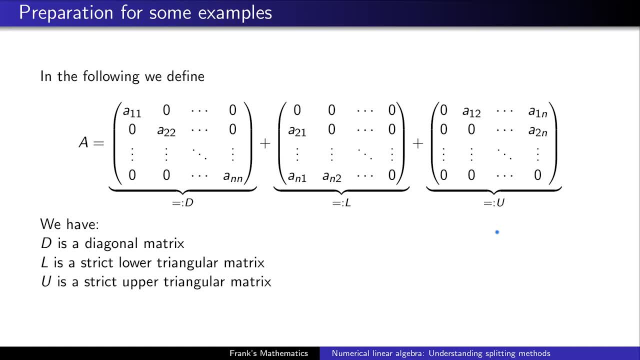 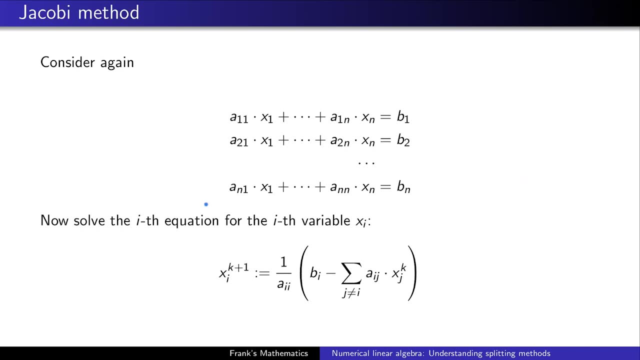 Keep this splitting Or keep this, Keep this, Keep this reformulation in mind, because this is very useful for analyzing the next algorithms. For our first algorithm, the so-called Jacobi method, consider again our n linear equations, now here in this full form. 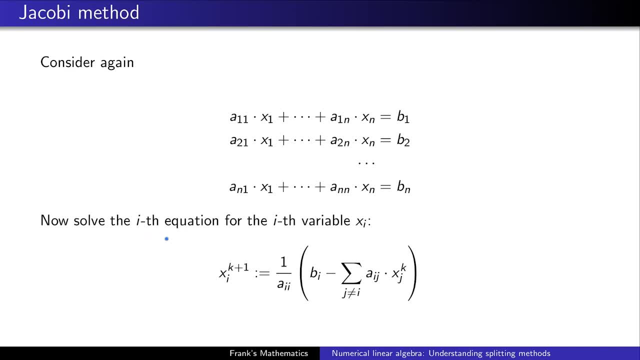 And the idea of the Jacobi method is OK. we take the i-th equation and solve it also for the i-th equation. So let's bring everything on the other side which does not contain xi And divide it by the coefficient of xi, which is aii. 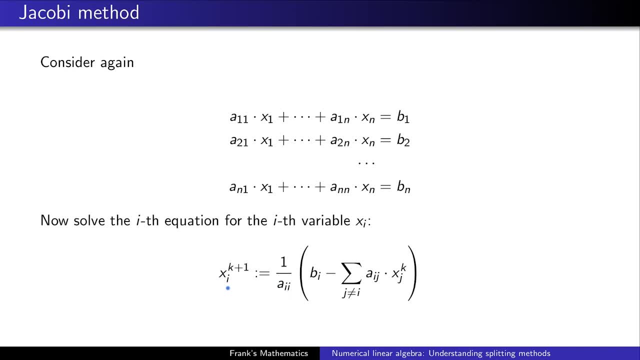 And call the resulting value xi k plus 1.. And do this for all i And you end up with a vector: x k plus 1.. This is the idea of the Jacobi method, And in the next slides I will tell you. 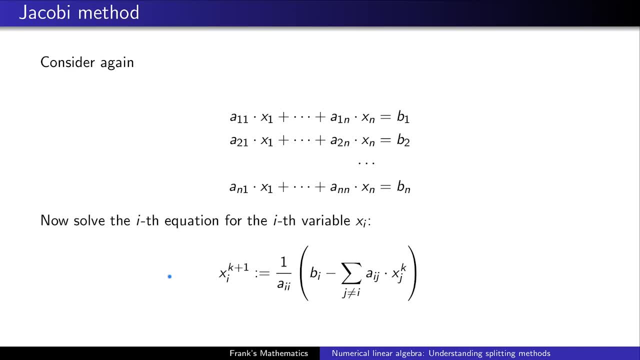 So, first of all, this is a very intuitive way of creating an algorithm: Just solve it. The idea is, if you have a triangular matrix, this is actually what you do. So if you assume that the matrix A is a lower triangular matrix, 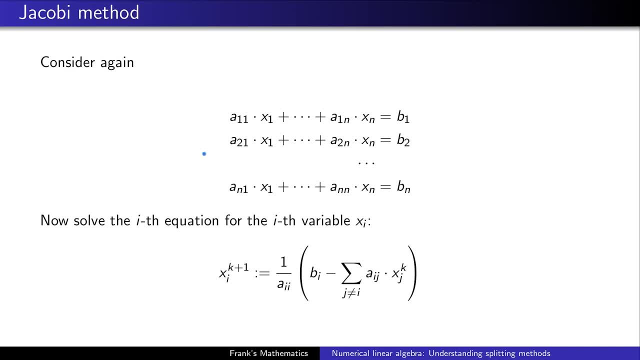 then this method here will give you the exact solution. So this is the idea of the Jacobi method, And in the following slides I will tell you, I will show you, how this can be reformulated into our setting, which will give us the general form. 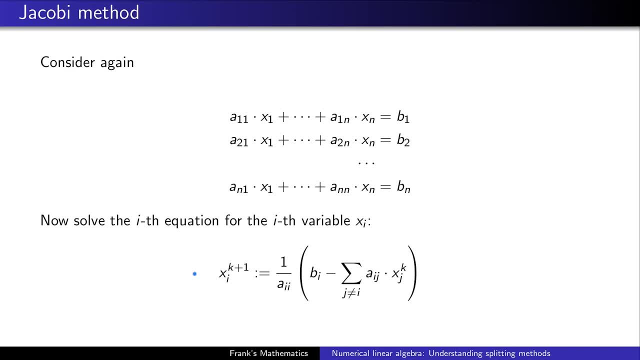 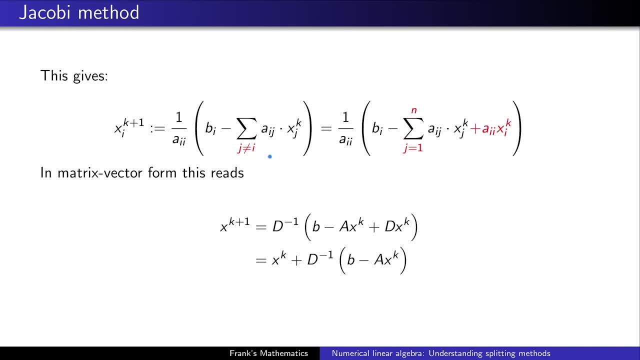 So, first of all, in our definition, in this sum, we do not have aii or xi containing, because this is excluded. Of course. it was brought to the other side, So just add it and subtract it again, So we have here a. 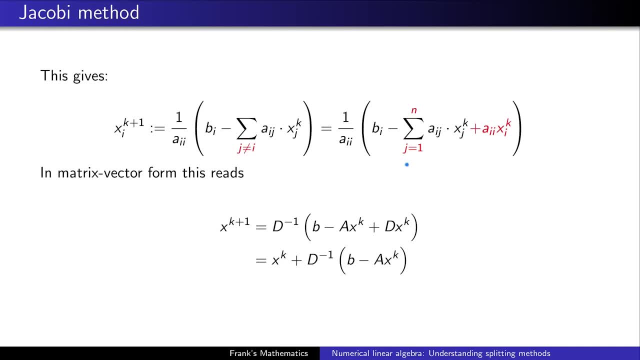 So a full sum kind of, Because this here is just the ith component of the vector a multiplied xk, And this value here is just the ith component of the vector d times xk. And if you made use of this, if you do this for all components, 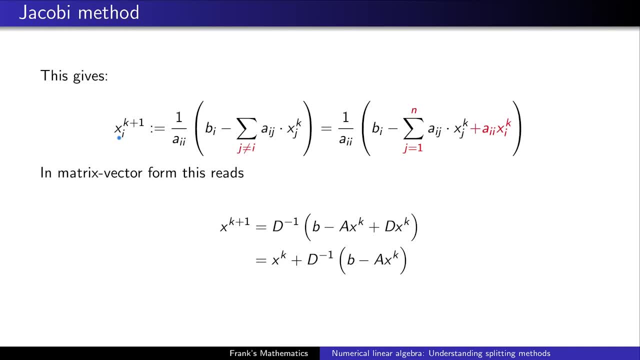 for all i, from 1 to n. you end up with this, You end up with this vector formulation here. So xk plus 1 is d, inverse of d, because inverse of d contains just element where d was a diagonal matrix, So it contains just the elements 1 over aii. 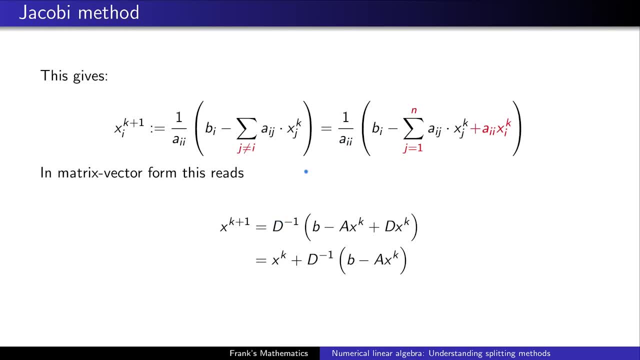 OK, for simplicity, we assume that the matrix d is of course invariable. bi will transform to b And already mentioned the second and this sum will give axk And this term, And here we'll give d times xk. 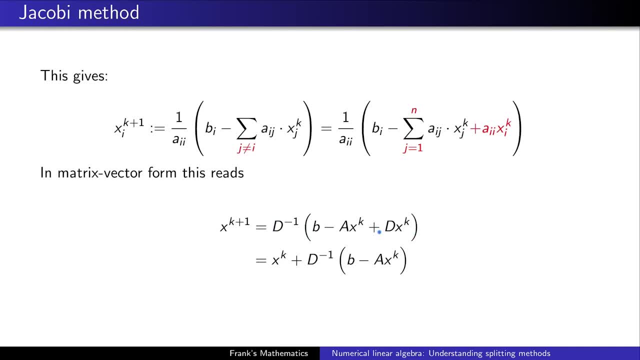 So this is nice, because now put d minus 1 into the sum And you will end up with this term here, And in fact this is all we have to do to get our Jacobi method into our general framework of the splitting method. 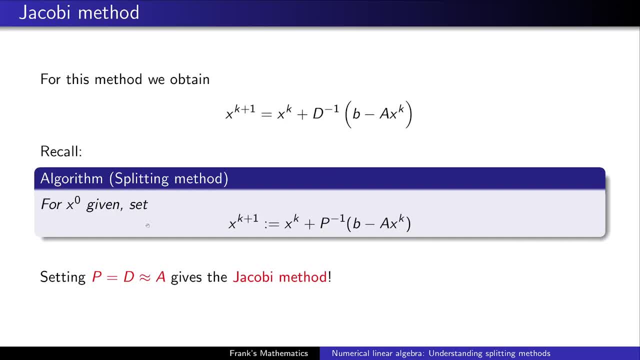 Because here you can see the splitting method again, Our splitting method was given this form, So here you have the Jacobi method. So if you set p to be the diagonal elements of the vector a, which is of course an approximation of a, 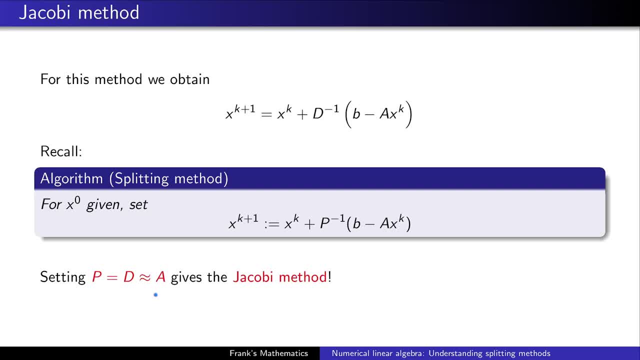 And it's very, very easy to invert. just invert the elements of the diagonal And the resulting method is called the Jacobi method. The Jacobi method works best if the elements of d are dominating, meaning that the elements that the diagonal elements of d are very big compared. 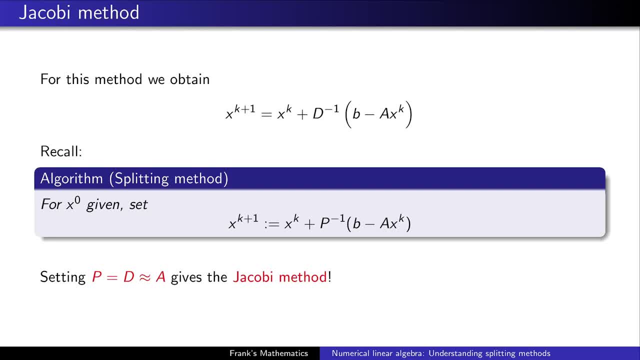 to the other elements of a. This is called a Jacobi method, This is called a diagonal-dominant matrix And this is used in the convergent analysis of the Jacobi method. But you can see that the easy choice of p to be equal. 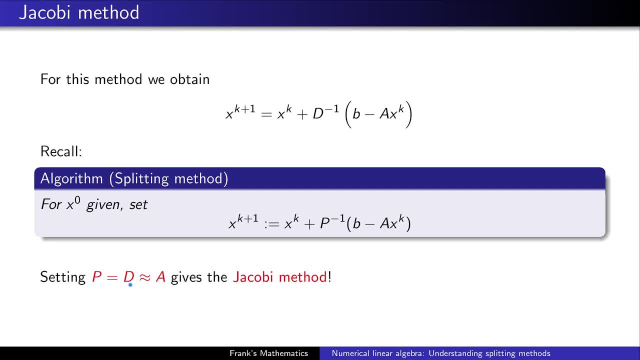 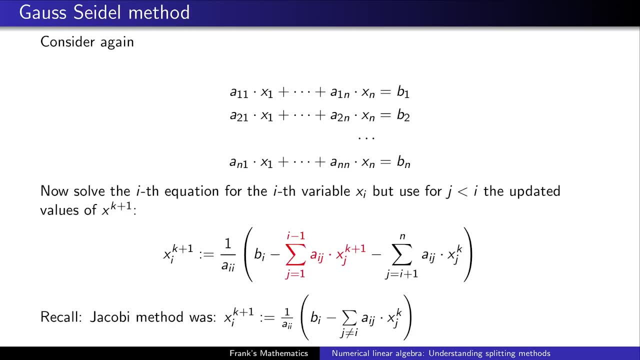 to the diagonal elements of a give a nice method. This is actually- I think this is- the first method you will learn in a school or in a university when it comes to splitting methods. The next method we want to take a look at is the so-called Gauss-Seidel method. 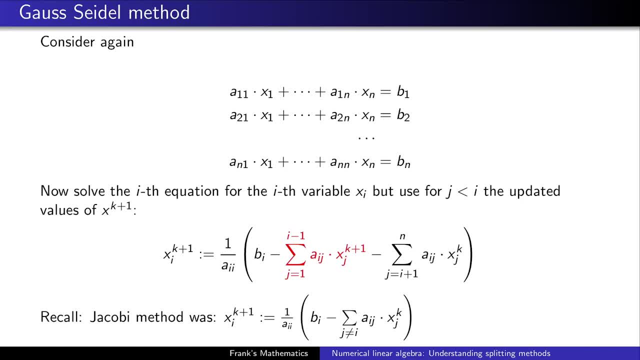 which is a PIMP version of the Jacobi method. Let's start again with our n linear equations. You can see them here And, again similar to the Jacobi method, we solve the i-th equation for the i-th variable, But instead of using the old vector. 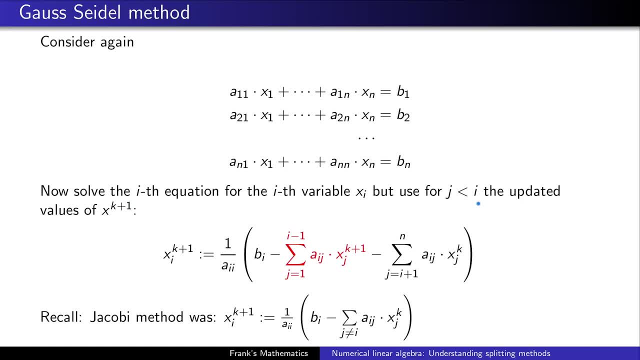 we use the updated vector for values j less than i. So what does this mean? Here you can see the Jacobi method And we have a sum here containing only elements of the vector xk, which is the old version. But if for j less than i, we already 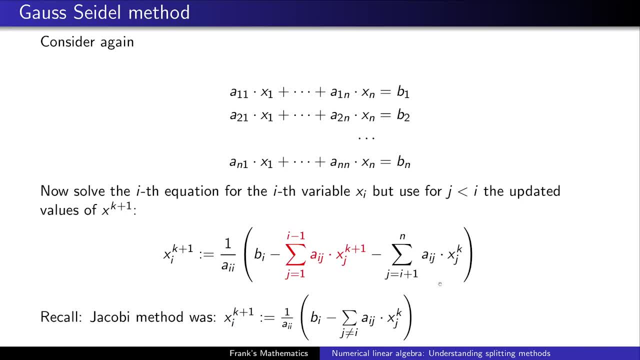 have the updated values of xk plus 1 at hand, because we computed them right here, so just use them. The idea is: the more information we have, the better the algorithm will be. This is the general idea, So let's split the sum into two parts. 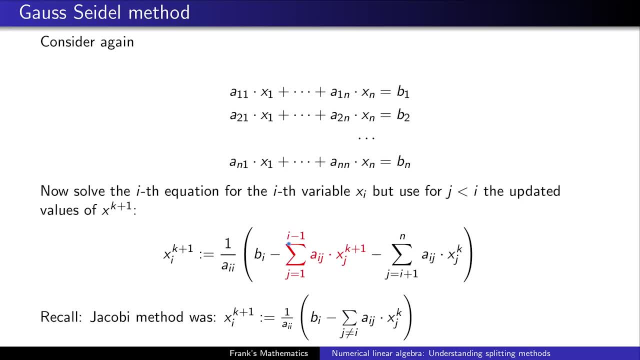 If you can see the first part here which contains for j less than i minus 1, contains element. So we have elements of the vector xk plus 1.. And here you can see the rest. So the sum is just split into old part and already updated. 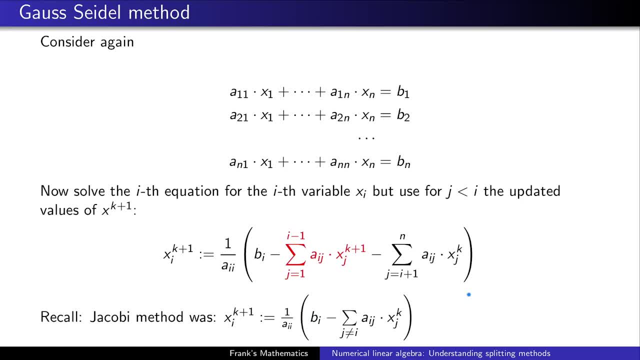 parts. Although this might look more complicated than the Jacobi method, when it comes to implementation it is way easier than the Jacobi method. Why is that so? For the Jacobi method, I have to store two vectors, the xk. 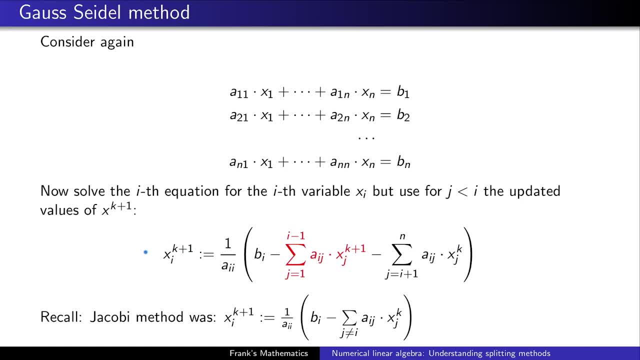 so the old version and the updated vector xk plus 1.. This is not needed here. You can store all values in just one vector, because if you have computed xk, xik plus 1, well, just write it into the same vector. 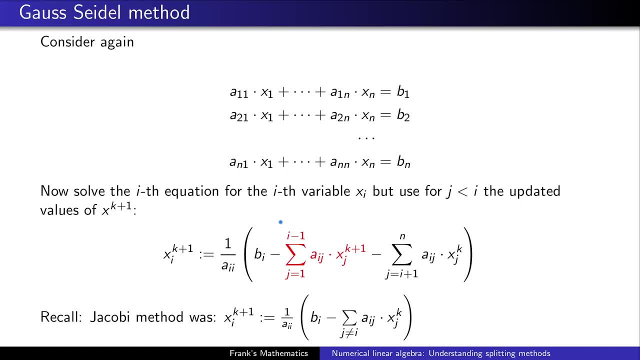 because we will use the old values here, So there is no need for storing it in a separate vector, which makes the implementation very easy. OK, can we put this method into our general framework? We can, but we have to do a little bit of work here. 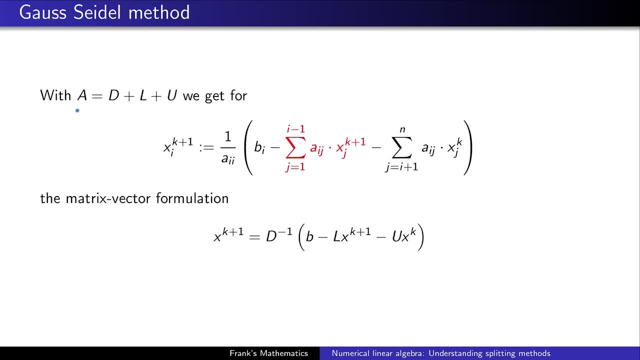 So let's do that. So we make heavy use of our splitting. a is d plus l plus u. Here you can see again the Gauss-Seidel method, And again we reformulate this as a matrix vector formulation. So this fraction, here we give, of course. 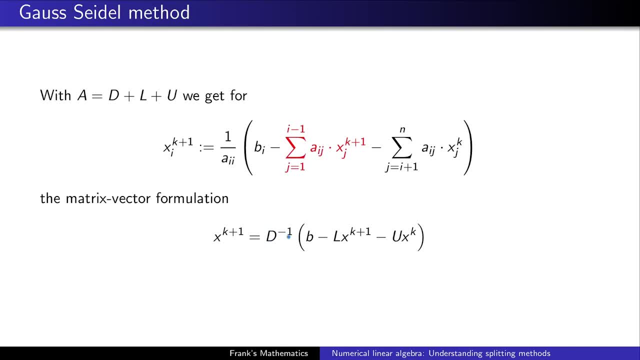 the inverse of d, which contains just the diagonal elements. The red sum here contains just elements of the lower part of l, of i, of a, of the matrix a. So this sum here, The red sum here, is exactly l which. 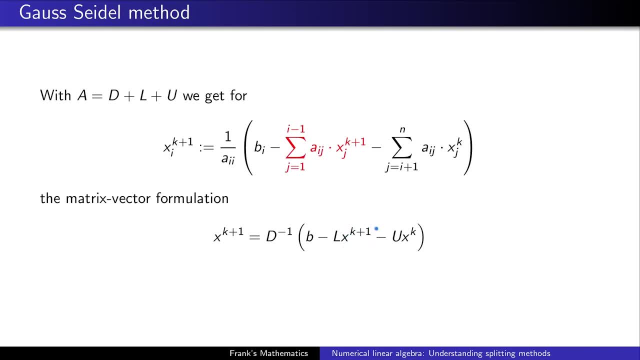 is a strict lower triangular matrix times xk plus 1, so the updated one, while the right-hand side, in a similar fashion, contains only element of the upper part of the matrix a. So this is just u times xk. 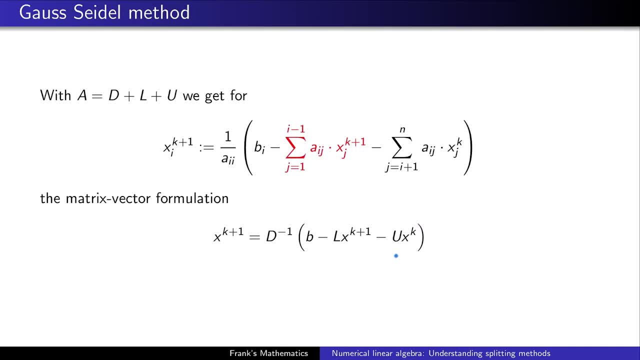 u contains the upper elements, the elements above the diagonal, if you remember it correctly. Now we have this matrix vector formulation at hand and we can reformulate it now to fit into our general framework. This is a little bit of a lengthy calculation. 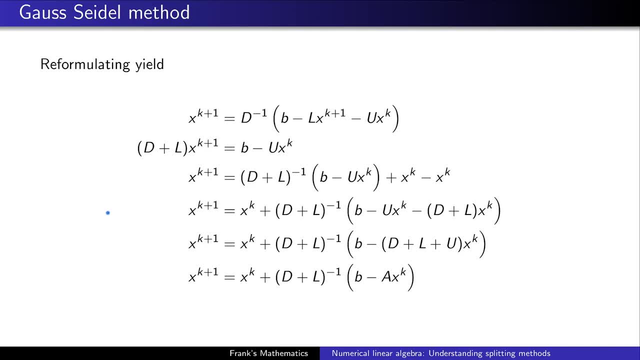 but I put it here into detail because there's a nice trick that I want to show it to you. Let's start with this equation here First. one first step is to bring d to the other side. So we have d times xk plus 1 on the left-hand side. 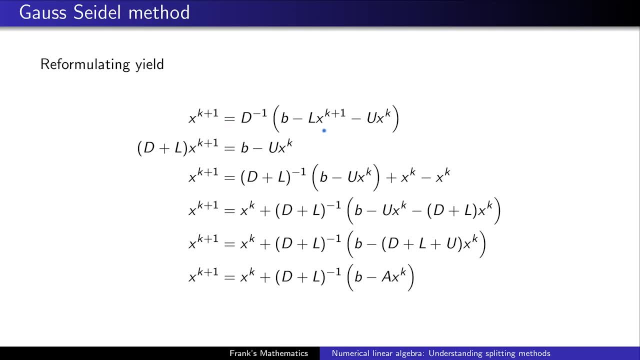 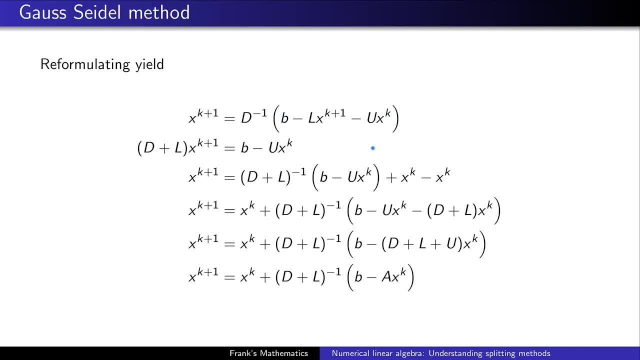 So this is what's left here on this side. Assume that d plus l is invertible, Bring it to the other side and you will end up with this term here And now. here's a little trick To get our thing into our setting. we want just add: 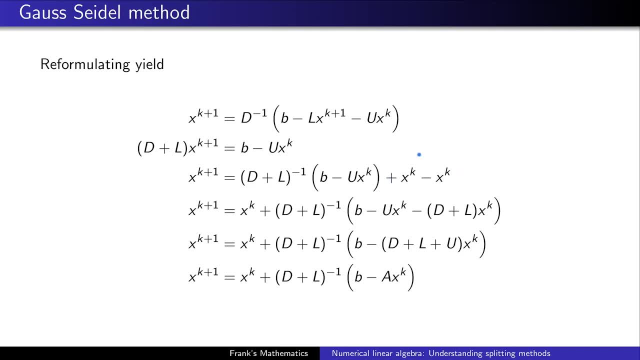 the stuff, add the vector we want and subtract it. So this is 0.. So we do not change the value of, do not change the equation here. So bring one xk in front and the other xk is brought into this equation here just by adding d plus l xk. 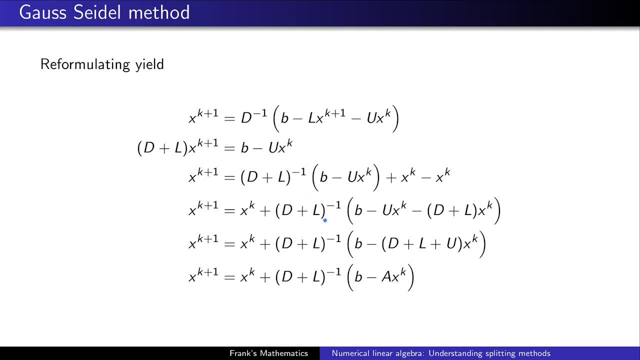 because this cancels out with the inverse here. Just bring it into the term here. But now this looks much more nicer, because what do we have here? We have d xk plus l, xk minus u, xk, So d plus l plus u, which is exactly a. 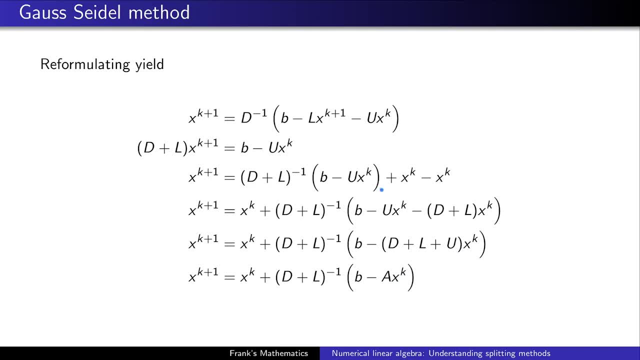 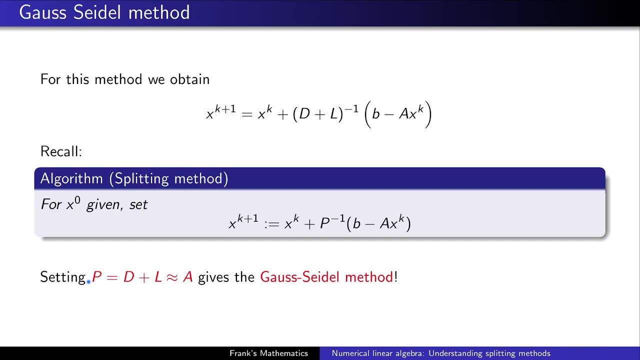 So using the adding and adding a 0, basically this is just adding a 0. This is called adding a 0. We have formulated our Gauss-Seidel method into our general framework, which allows us now to see that, if you choose p to be the diagonal matrix, 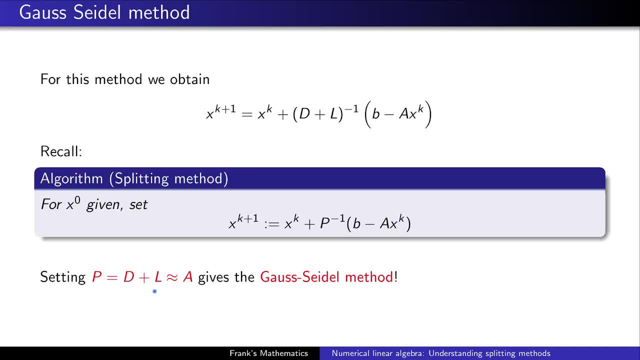 plus the lower part of the matrix l, we end up with the Gauss-Seidel method Again. compare it here. And of course d plus l is a much better approximation of a than just the diagonal elements which it was for the Jacobian method. 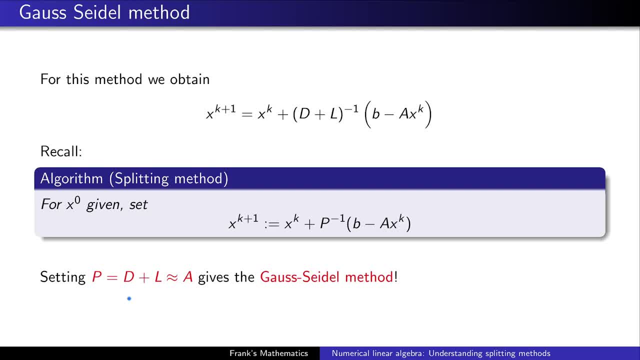 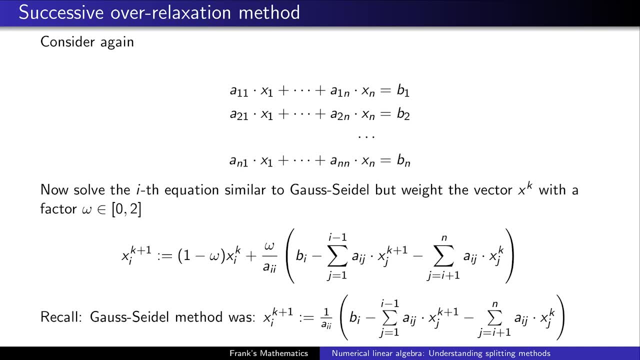 So, in fact, this is a Much more better method than the Jacobian method, of course. Third and the last method I want to show you is the so-called successive over-relaxation method, or SOR method, which actually includes the Gauss-Seidel method. 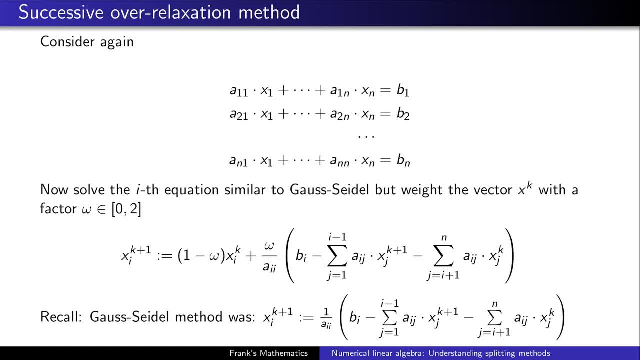 as a special case. So again, here we have our linear equations. We solved the IF equations, similar to Gauss-Seidel, But now, in order to speed up the conversion speed, we add a combination of the old vector xk with the outcome of the Gauss Seidel method. So you can see: 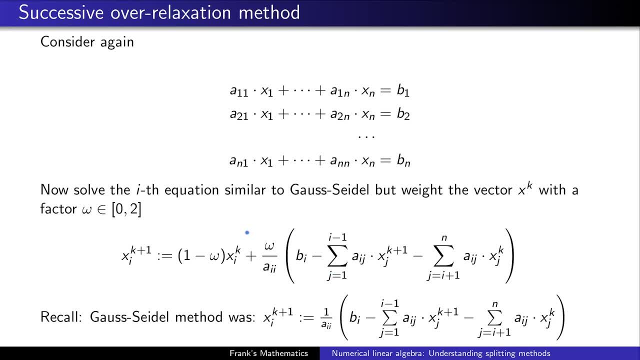 we have to term coming from Gauss Seidel And we add the combination of the old vector. so I minus omega, times xk plus omega and the outcome of the Gauss Seidel method. So if you choose omega to be one, well, we basically end up with the Gauss 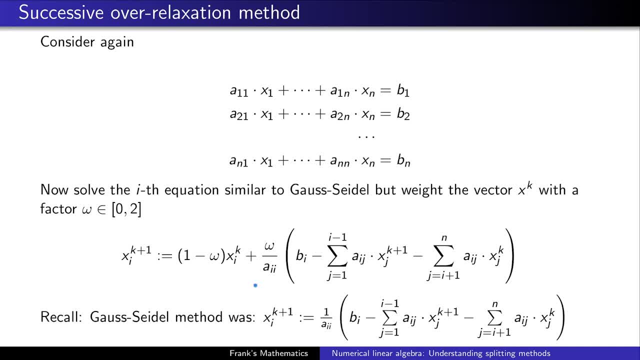 Seidel method. So this is a kind of extension of the Gauss Seidel method, and omega has to be chosen correctly And there exists a lot of analysis for this: how to choose omega correctly In order to get the fastest conversion speed. Can this be put into our, our framework? I mean it can of 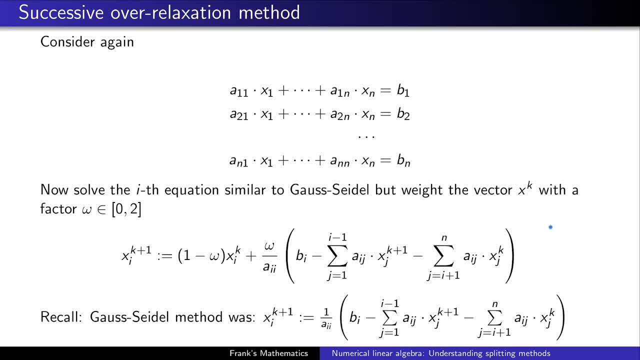 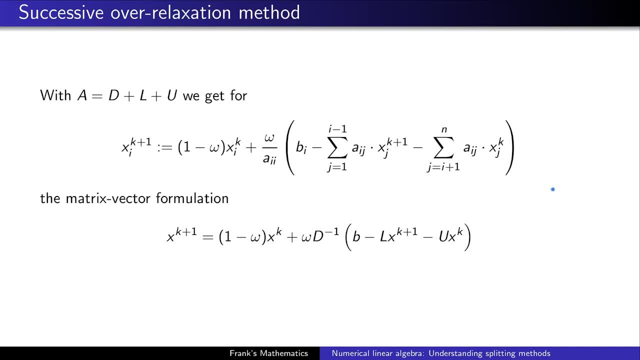 course, I will just rush through it, because the calculations do not differ that much. Again, we use our splitting. here you can see the SOR formulation And if you put it into a matrix vector formulation, you basically end up with: this: is the term coming? 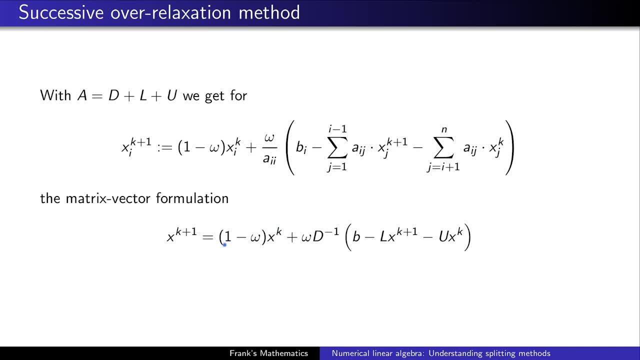 from Gauss Seidel, And this, of course, will give us one minus omega times xk. Do a lot of calculations And you'll end up with this term is xk plus one, is xk plus omega times d plus omega L, inverse. Again, if you choose omega to be to be equal, one will. 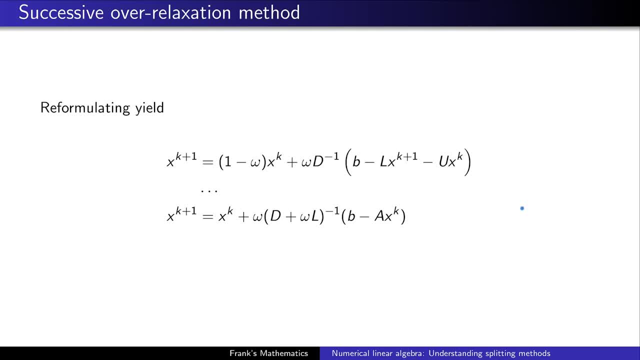 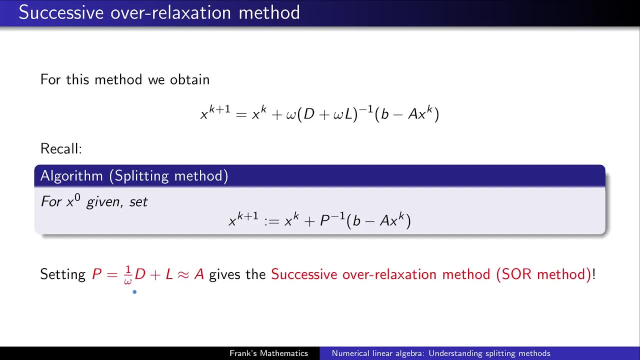 end up protect me with the Gauss Seidel method. So, in terms of our splitting method, if we choose P to be chosen as one over omega d plus L, this gives us the SOR. this will give us the SOR method. So the idea is here is to put a weight on the diagonal. 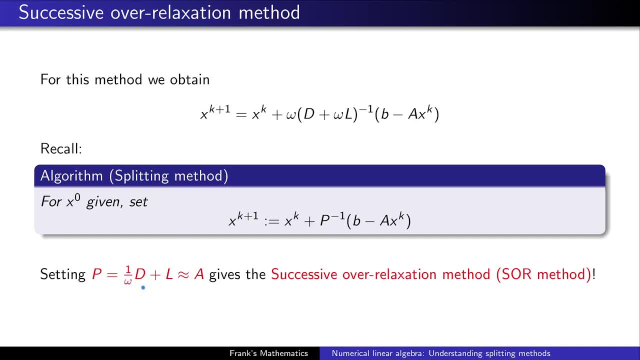 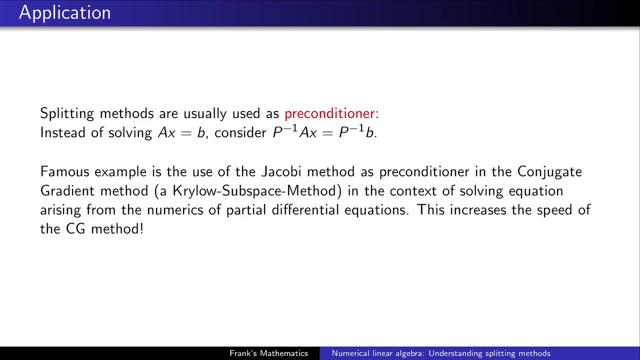 matrix. This is the idea of the successive over relaxation And you can see it here in the approximation formulation of our matrix P. We have not talked a lot about how to put splitting methods into general frameworks and do a lot of calculations. But what are they actually used for? And mostly splitting. 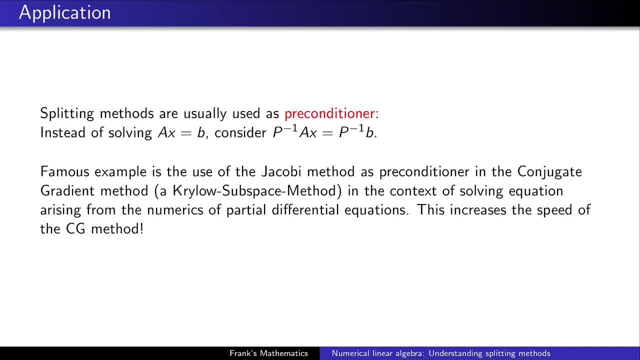 methods are used as preconditioner, meaning we want to solve ax equals B, But instead of solving ax equals B, we solve P minus one. ax equal P minus one B. So we reformulate the system And again P should be chosen as: 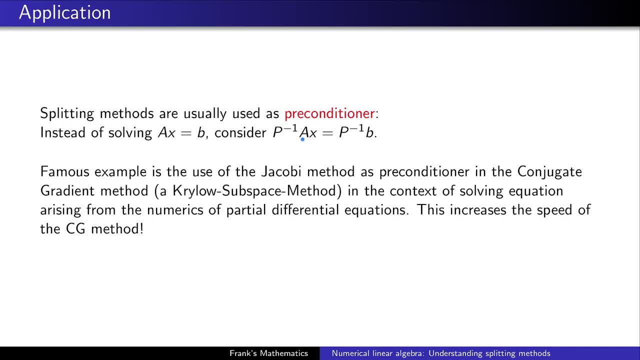 a buffer as a good approximation of the matrix A, And a famous example is, for instance, the use of the Jacobian method as a preconditioner in the conjugate gradient method In the context of solving equations, which comes from a matrix of partial 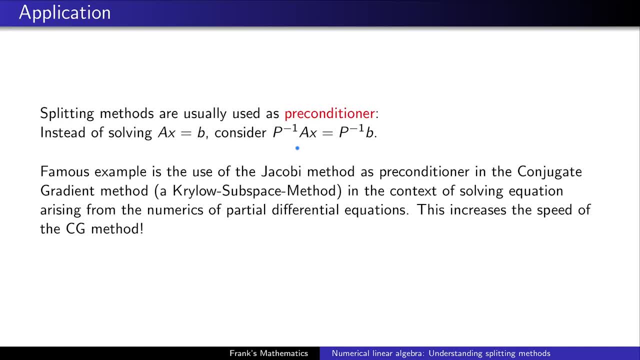 differential equation. The matrix there has a very specific form which makes it very suitable for for preconditioner, For instance the Jacobian method, And this increases the speed of the conjugate gradient method a lot. I think I will do a video about this, about this.